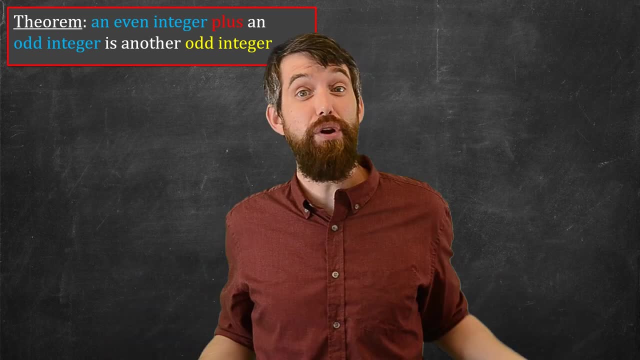 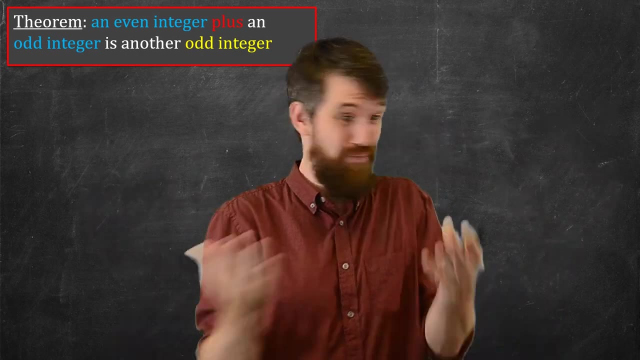 and it adds up to 5,, which is another odd. Now that seems straightforward, but are you 100% convinced that this theorem is true? for every possible way, you can do it. every possible way, you can add an even to an odd. And, more importantly, if I'm a skeptic, could you convince? 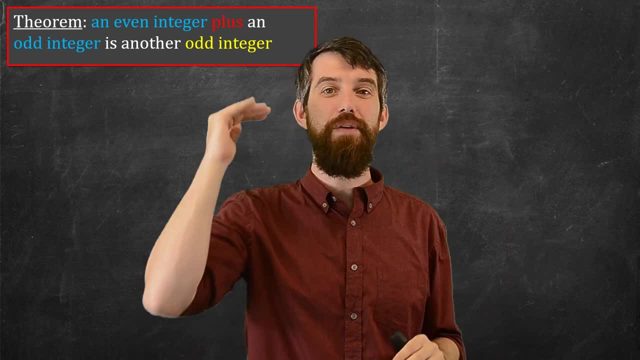 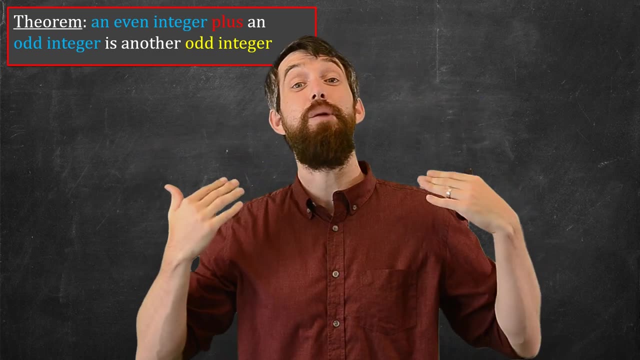 me of that. So this is the point of this video. I'm going to show you the basic scaffolds for how you can do a formal, direct proof, how you can get started and how you can complete it. The actual theorem doesn't matter so much, It's just a particular example of the structure. 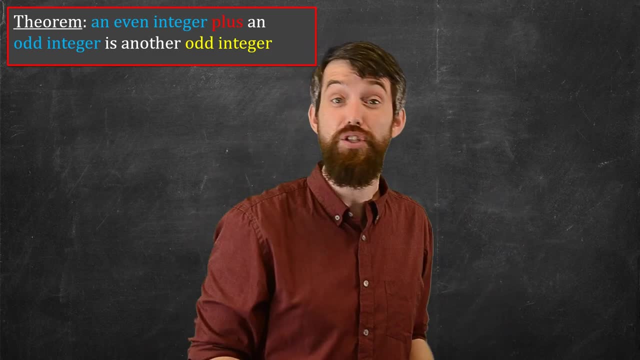 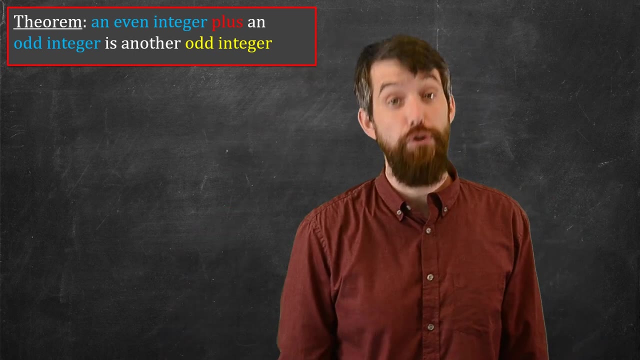 of a simple direct proof, And then we're going to go on This course. we're going to see all kinds of different formal proofs of all kinds of different claims. OK, so let's get started on actually proving this. The first thing: 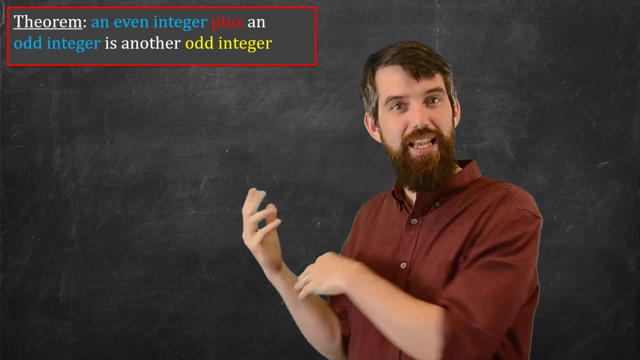 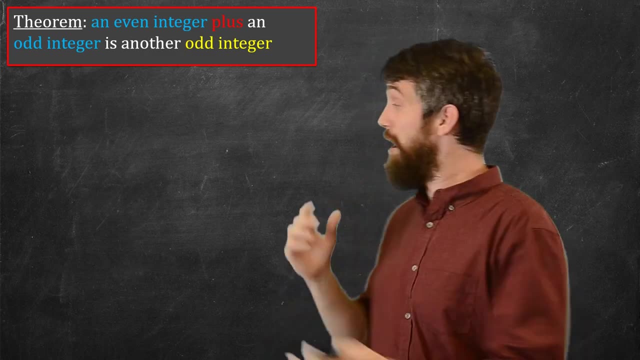 I want to do is that I want to be precise about what we're actually saying here and what my definitions are. And in the previous video we saw the definition of being even and being odd. And there they are. We would say that an integer n was even if there was. 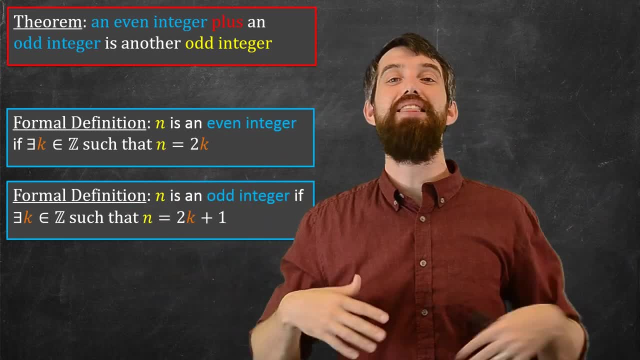 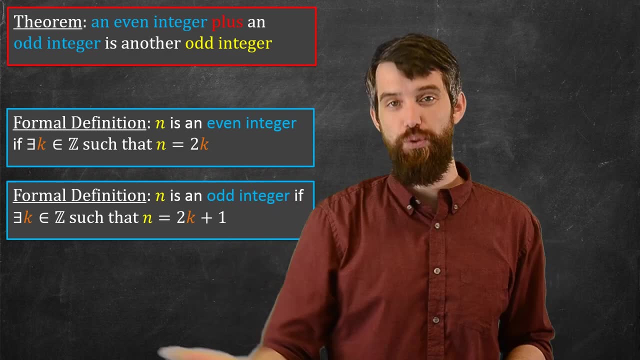 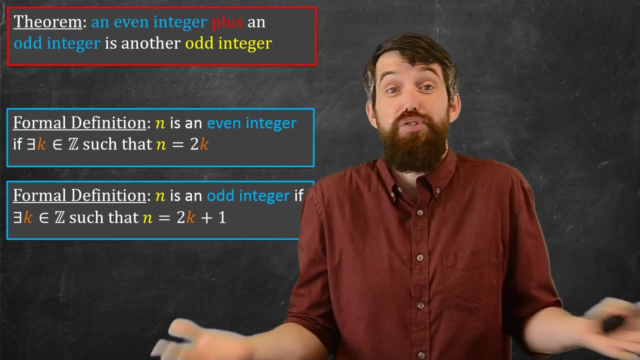 some other integer k where n was twice k And we'd say that an integer n was, even if n was odd, if there was some other integer k such that your n was twice k plus 1.. So these are the two major words that are sort of mathy in this particular theorem And before you. 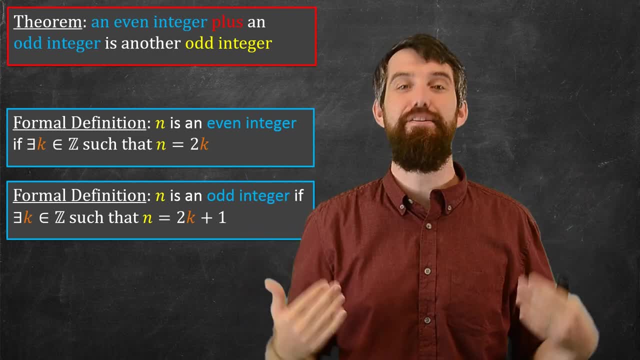 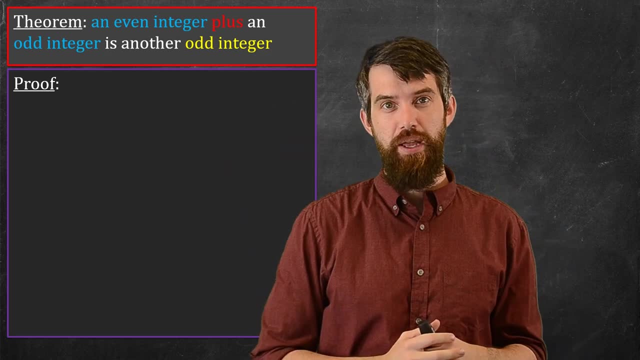 even get started proving any theorem, you have to have a precise definition of the concepts that are in that particular theorem. All right, So now let's try to prove this particular claim. Now, the first thing I want to note is this: This claim is written in the form 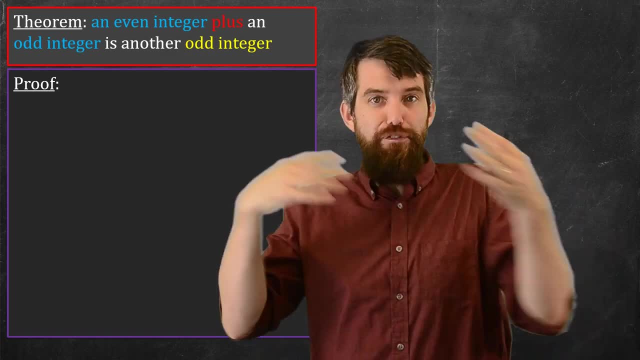 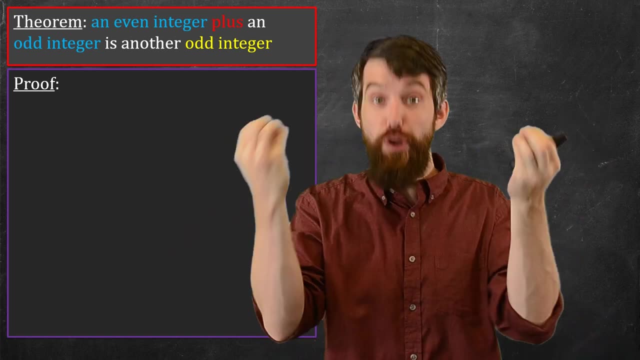 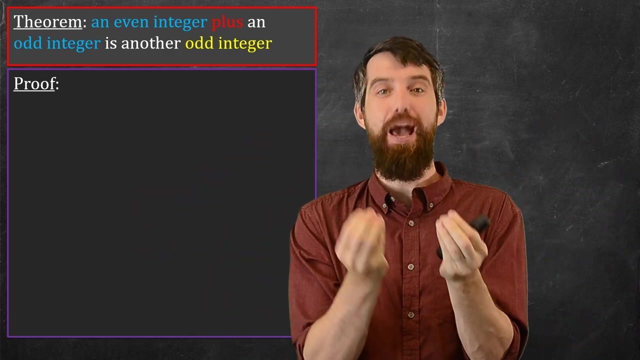 of: if p, Then q. It says if you have some assumptions, namely you've got an even integer and an odd integer, then you get a conclusion that the sum of those two things is an odd integer. So it's saying: if you've got an m and an n, that's even and odd. then you add the m and. 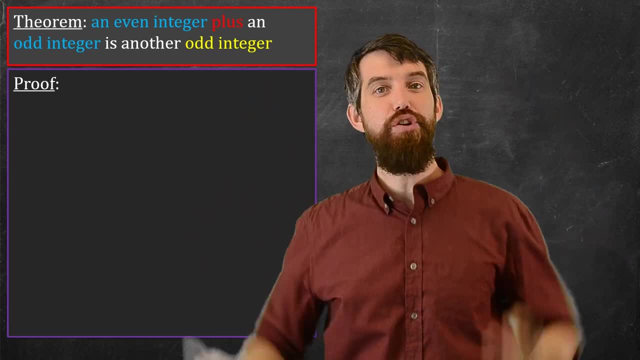 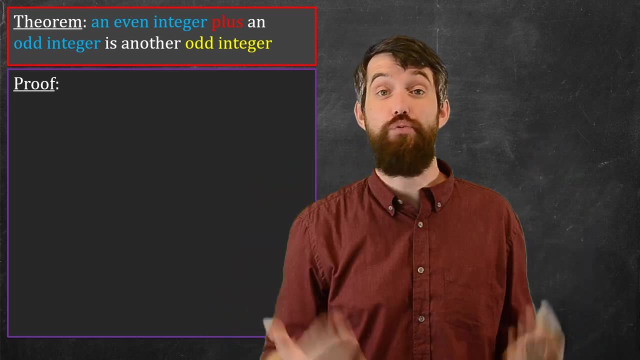 the n and you get an odd. So when I want to do this proof- if it goes, if some assumptions, then a conclusion- my proof should follow that basic logic. when I'm doing a direct proof, I want to begin with the assumptions. 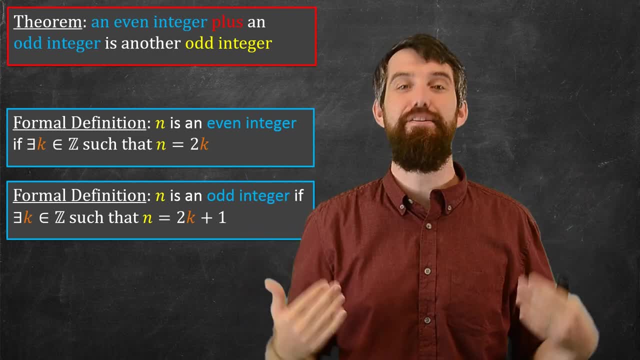 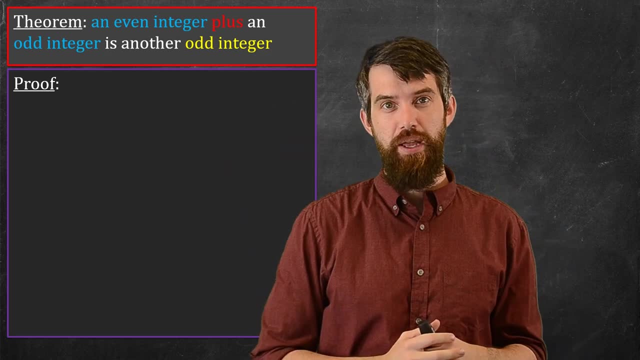 even get started proving any theorem, you have to have a precise definition of the concepts that are in that particular theorem. All right, So now let's try to prove this particular claim. Now, the first thing I want to note is this: This claim is written in the form 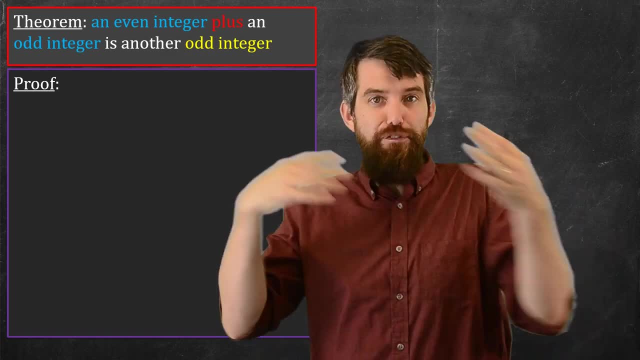 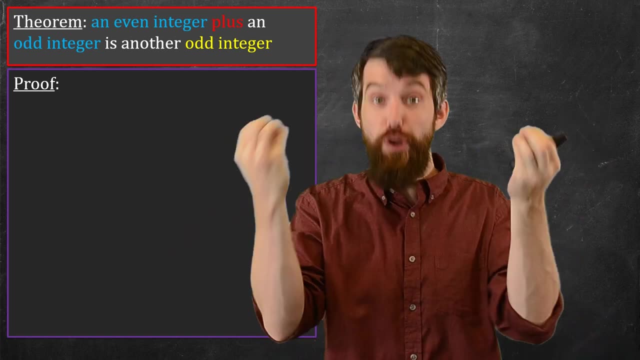 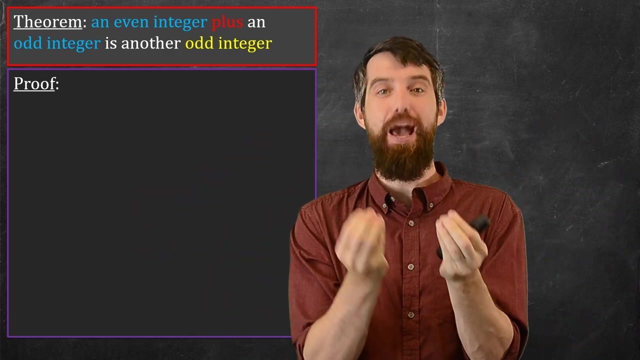 of: if p, Then q. It says if you have some assumptions, namely you've got an even integer and an odd integer, then you get a conclusion that the sum of those two things is an odd integer. So it's saying: if you've got an m and an n, that's even and odd. then you add the m and. 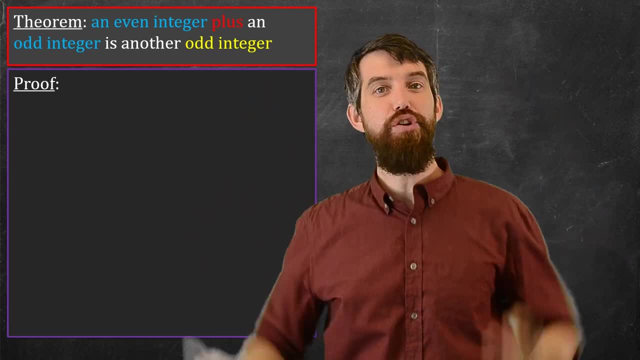 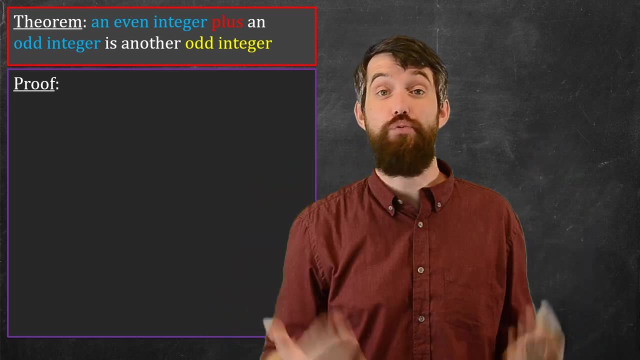 the n and you get an odd. So when I want to do this proof- if it goes, if some assumptions, then a conclusion- my proof should follow that basic logic. when I'm doing a direct proof, I want to begin with the assumptions. 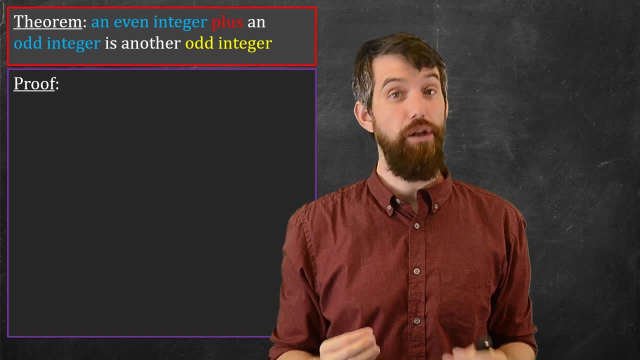 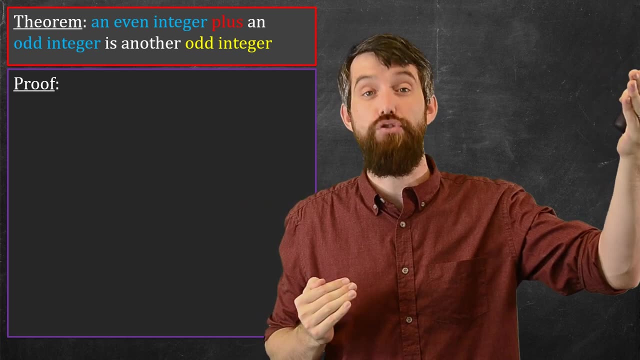 I'm going to go on and follow some process and then I'm going to end with the conclusion, And so when you read it, everything makes sense. You start with what you're supposed to assume and you do various manipulations and you get to what you're trying to conclude. 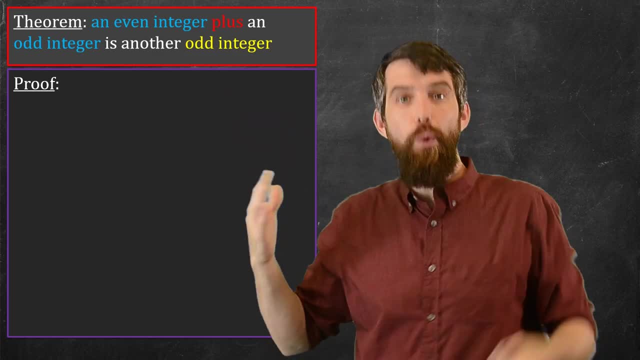 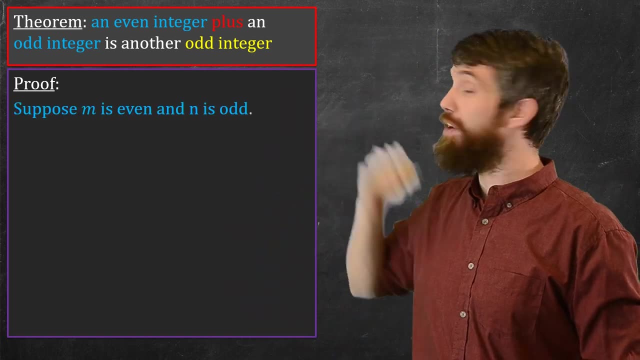 That is how you do a direct proof. So in this case, well, what's my assumption? It's the m is even and that the n is odd, and that's what I'm going to begin with. So that's going to be my very first line of my proof: Let m be even and n be odd. 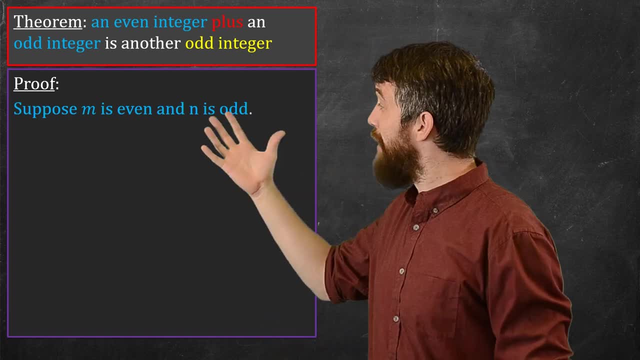 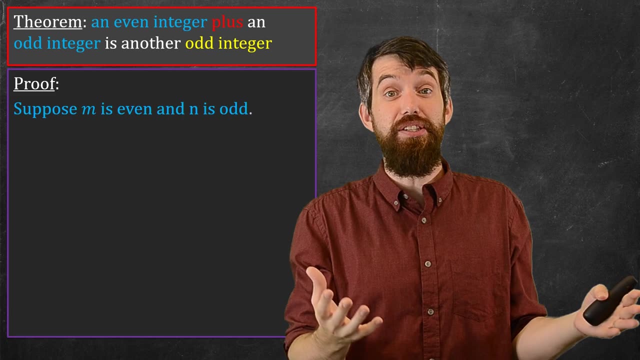 All right Now. the problem right now is that the m being even and the n being odd is going to be a little bit imprecise, But thankfully we've already defined the precise notion of what it means to be even and odd. To be even, it says that there is some integer k such 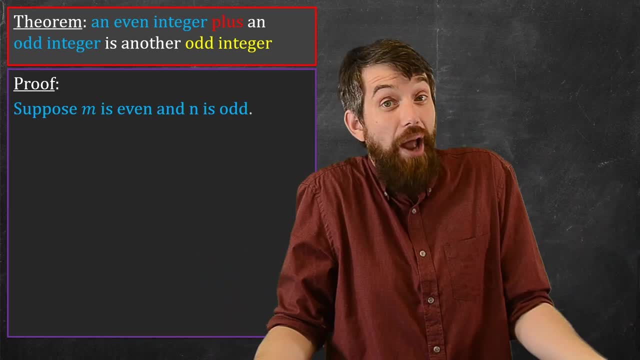 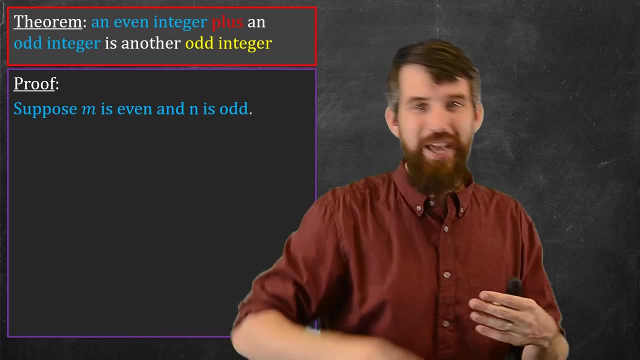 that m can be written as twice k And, to be odd, it means that there is some other integer k, so that n can be written as twice k plus 1.. However, because I've got two different numbers here, the m and the n, you get two different k's. I'm going to actually call. 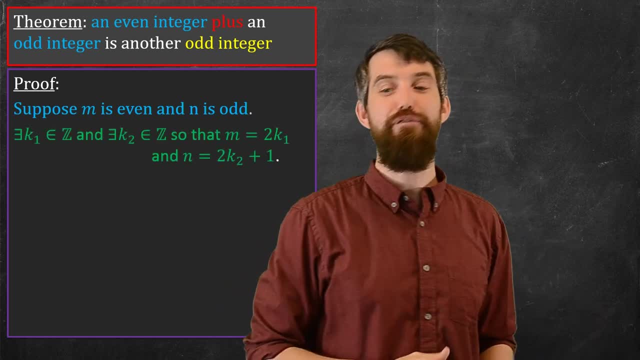 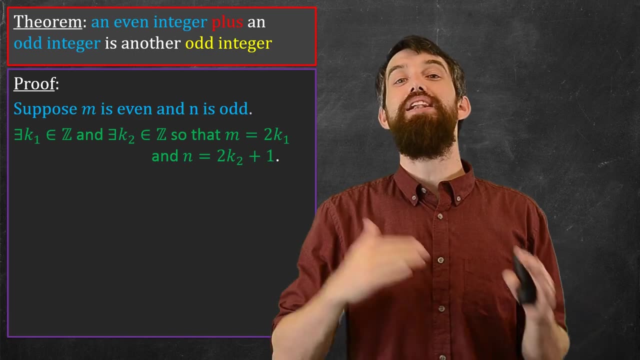 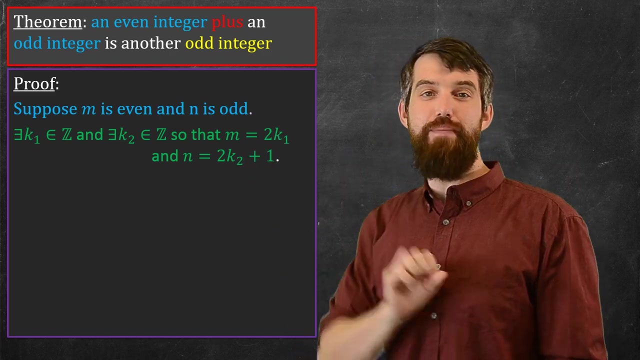 them k1 and k2.. And so when I apply my formal definition, here it is, It says there is an integer k1 and there is another integer k2.. And that is what lets you write m as twice k1 and n as twice k2 plus 1.. So this is the precise mathematical definitions of being even and. 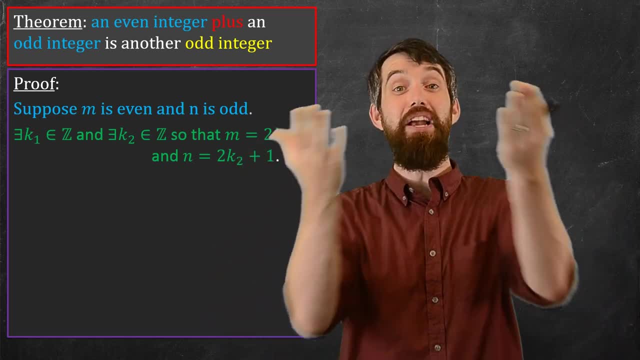 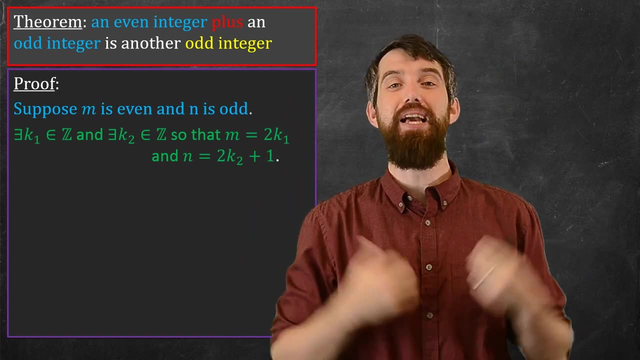 odd. Now, why do I care about this? Because now I can plug these into formulas. In particular, the theorem that I have here asks for the sum of these two things. I'm trying to make a claim about the sum of m and k. 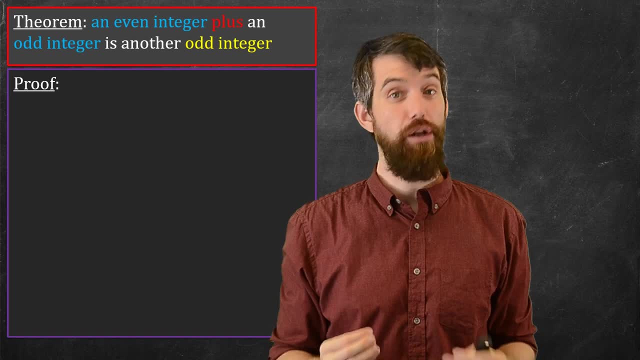 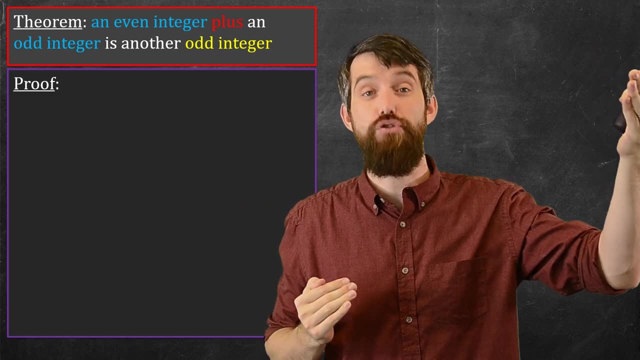 I'm going to go on and follow some process and then I'm going to end with the conclusion, And so when you read it, everything makes sense. You start with what you're supposed to assume and you do various manipulations and you get to what you're trying to conclude. 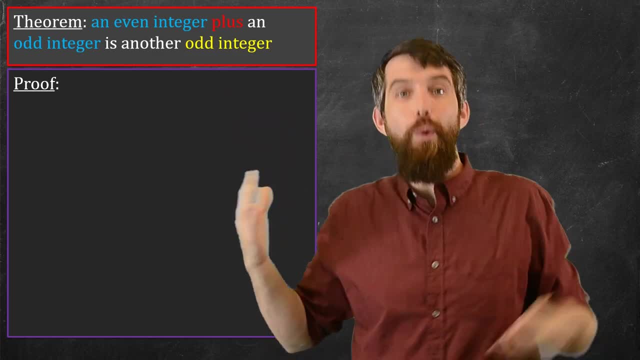 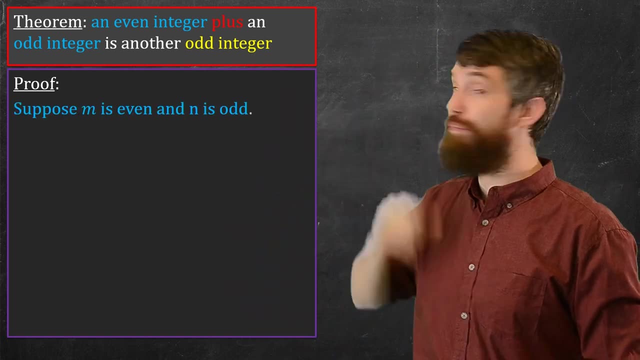 That is how you do a direct proof. So in this case, well, what's my assumption? It's the m is even and that the n is odd, and that's what I'm going to begin with. So that's going to be my very first line of my proof: Let m be even and n be odd. All right, Now the 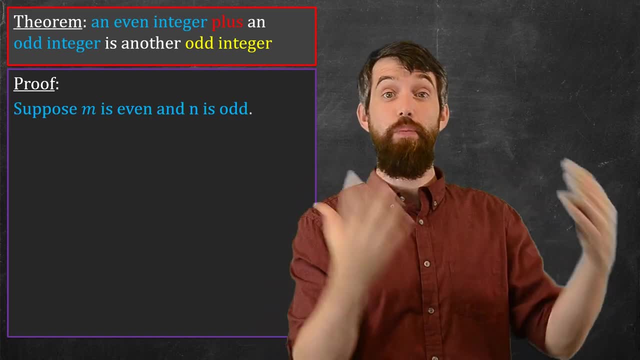 problem right now is that the m being even and the n being odd are two different things. So what I'm going to do is I'm going to start with my first line of my proof. Let m be even and the n being odd is still a little bit imprecise, But thankfully we've already defined. 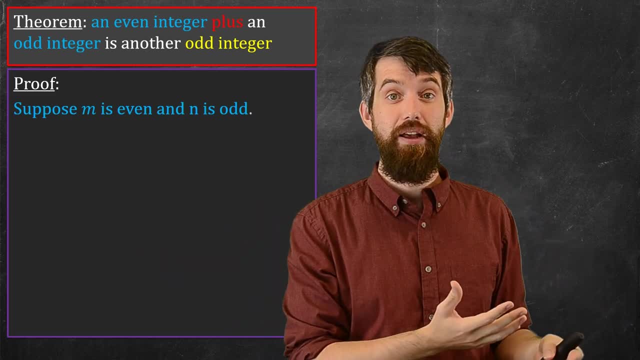 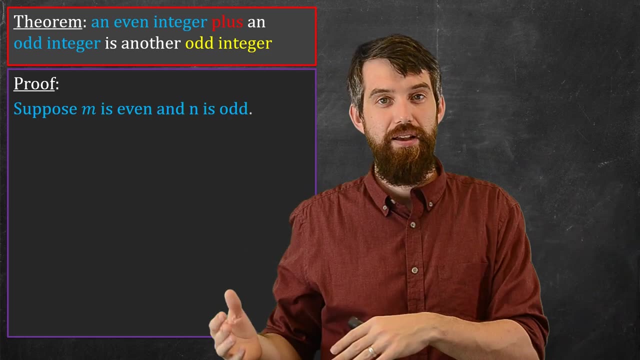 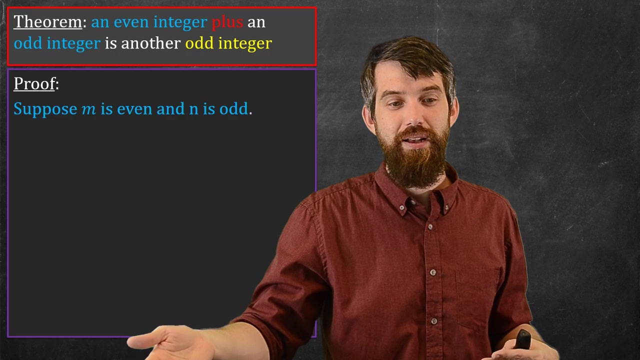 the precise notion of what it means to be even and odd. To be even, it says that there is some integer k, such that m can be written as twice k. And to be odd, it means that there is some other integer k, so that n can be written as twice k plus 1.. However, because I've got 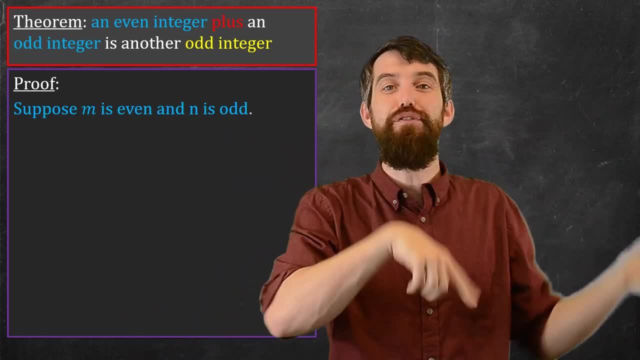 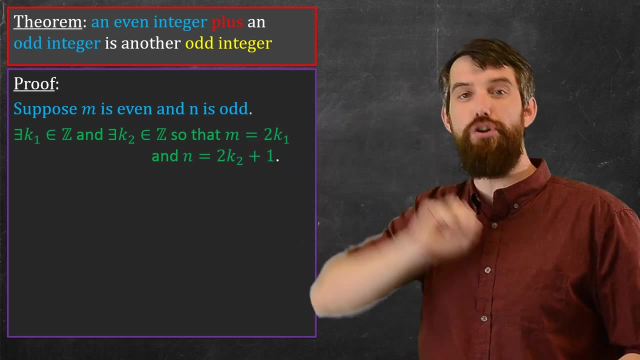 two different numbers here, the m and the n. you get two different k's. I'm going to actually call them k1 and k2.. And so when I apply my formal definition here it is, It says there is an integer k1. 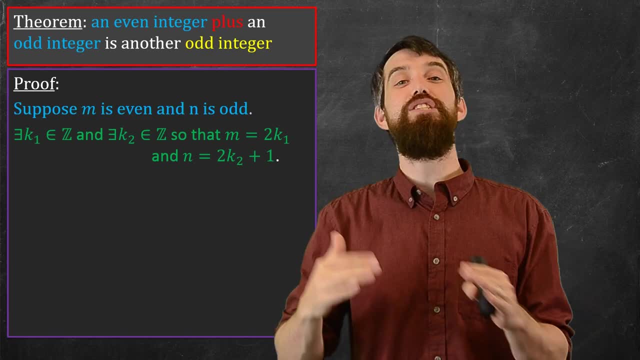 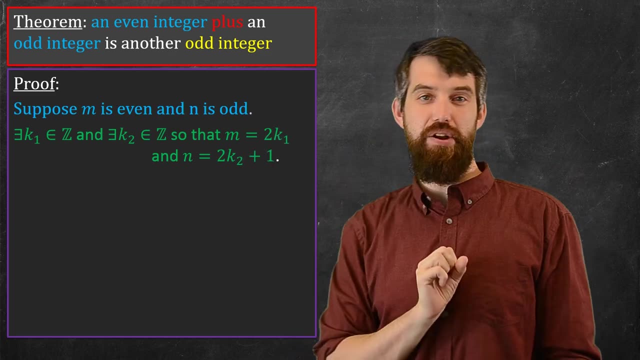 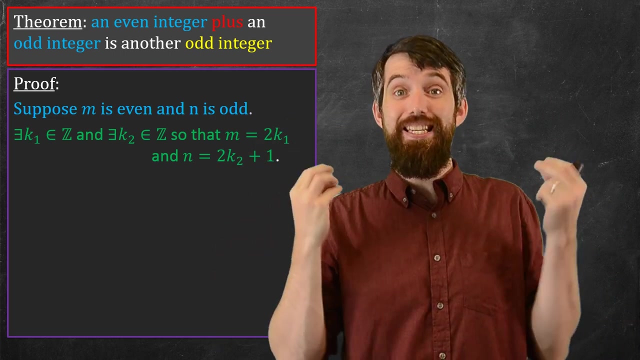 and there is another integer, k2.. And that is what lets you write m as twice k1 and n as twice k2 plus 1.. So this is the precise mathematical definitions of being even and odd. Now, why do I care about this? Because now I can plug these into formulas. In particular, 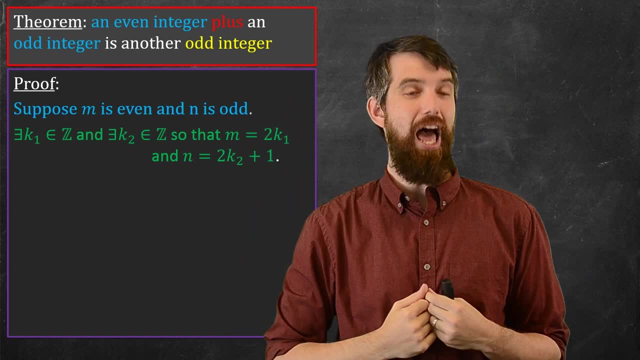 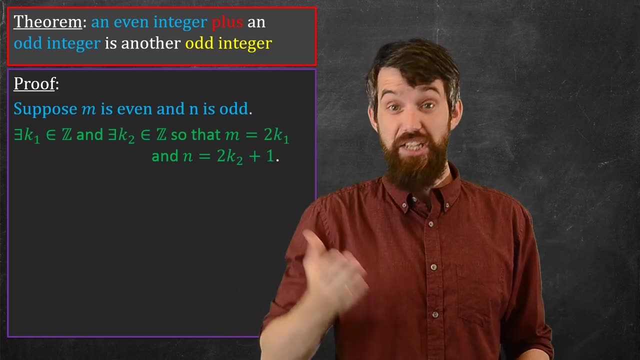 the theorem that I have here asks for the sum of these two things. I'm trying to make a claim about the sum of these two things, The sum of m plus n. So I'm going to take the sum of m plus n and I'm going to substitute: 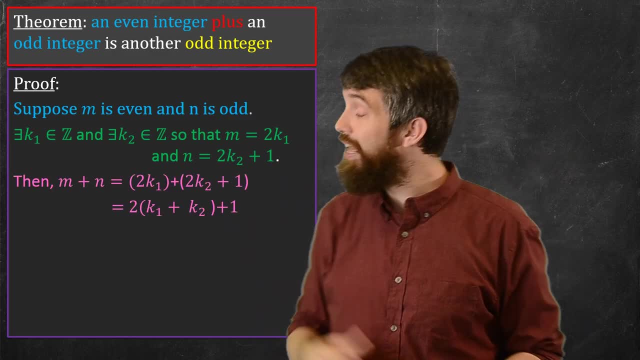 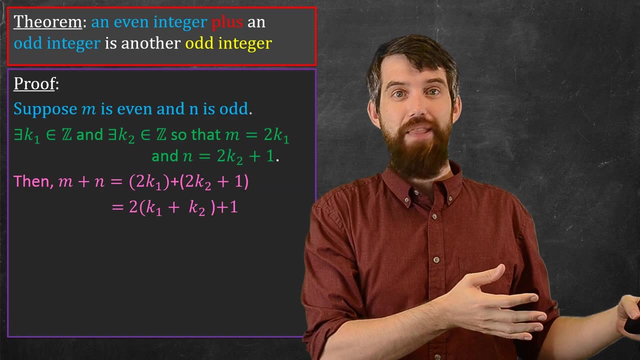 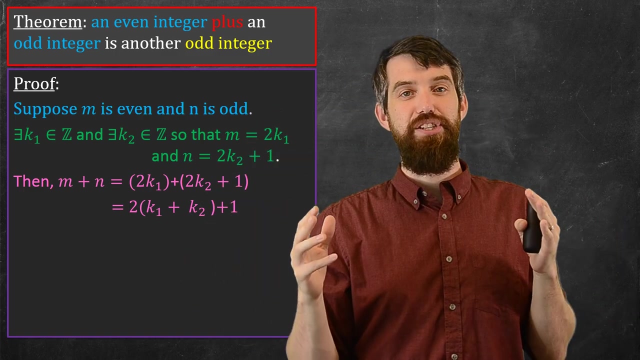 in precisely these definitions. So what do I get? I get m plus n. here is twice k1 plus twice k2 plus 1.. And then if I do this little bit of manipulation, I can bring a 2 out of the factors. I can say this is twice times k1 plus k2 plus 1.. 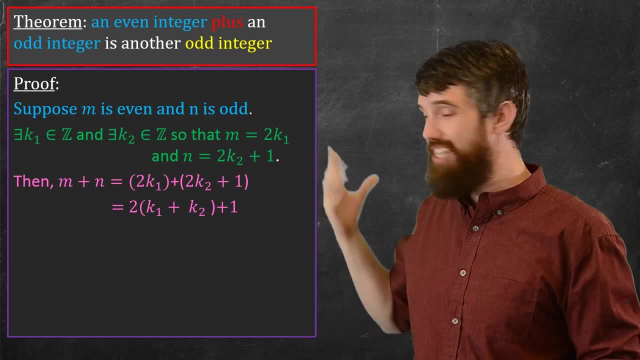 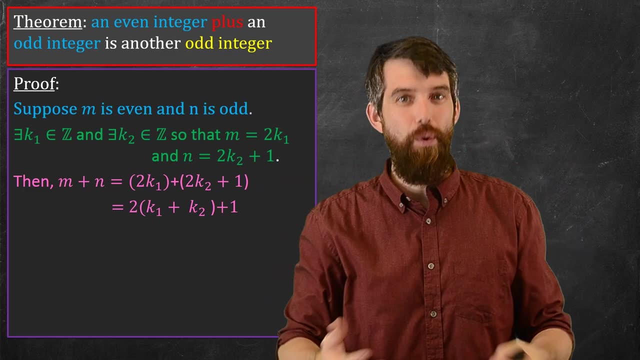 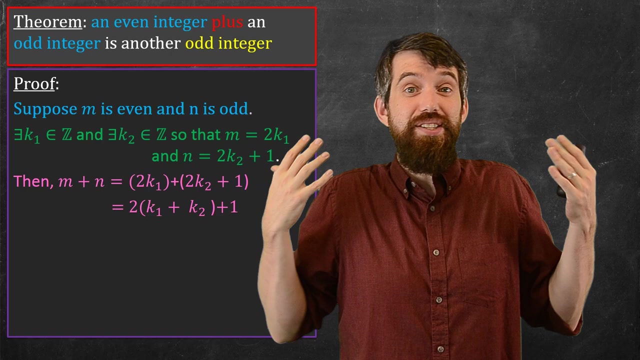 So basically I just applied my definition here to the sum And then I just did a little bit of algebra. Now why did I do the bit of algebra? What I'm trying to do, where I'm going, is that I want the sum of m plus n to be an odd integer. So I want the sum of m plus n to be written. 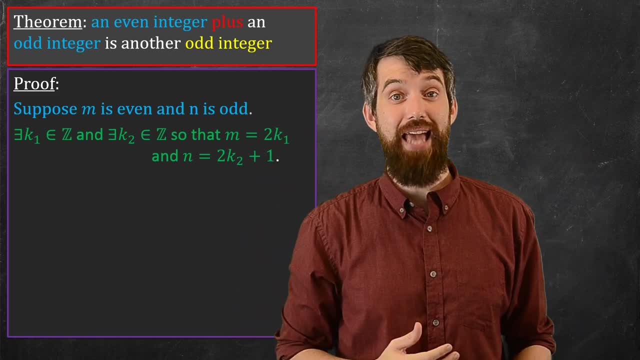 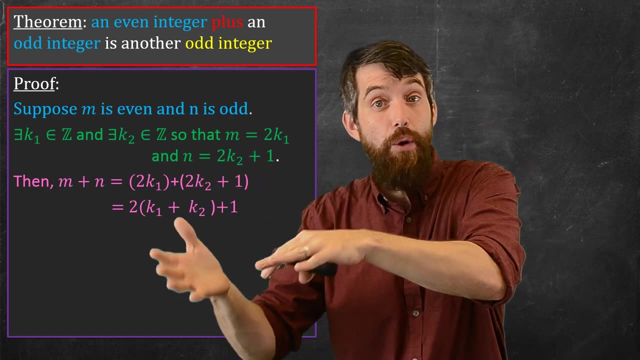 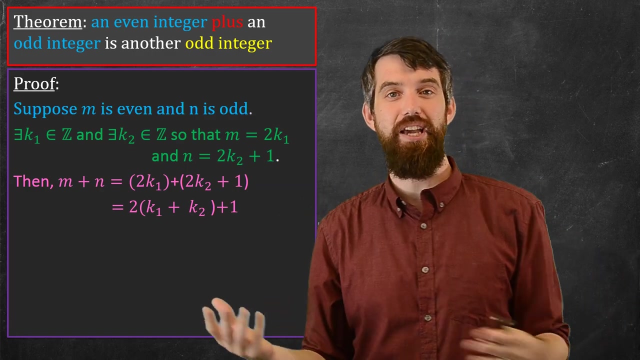 So I'm going to take the sum of m plus n and I'm going to substitute in precisely these definitions. So what do I get? I get m plus n here is twice k1 plus twice k2 plus 1.. And then, if I do this little bit of manipulation, I can bring a 2 out of the factors I can. 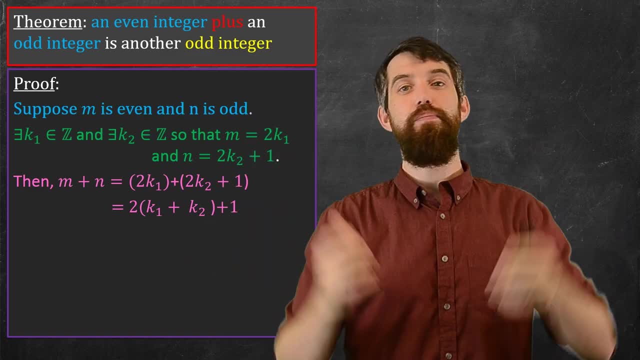 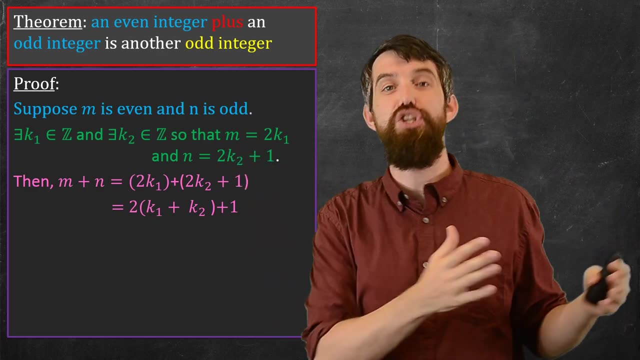 say, this is twice times k1 plus k2 plus 1.. So basically I just applied my definition here to the sum and then I just did a little bit of algebra to pull a 2 out of it. Now, why did I do the bit of algebra? What I'm trying to do, where I'm going, is that 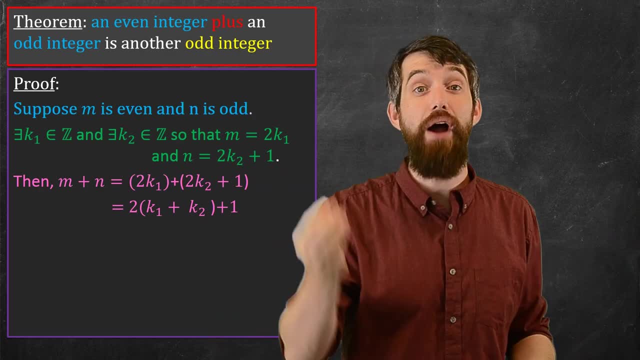 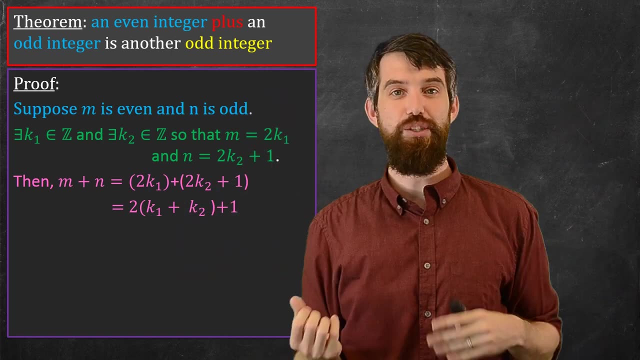 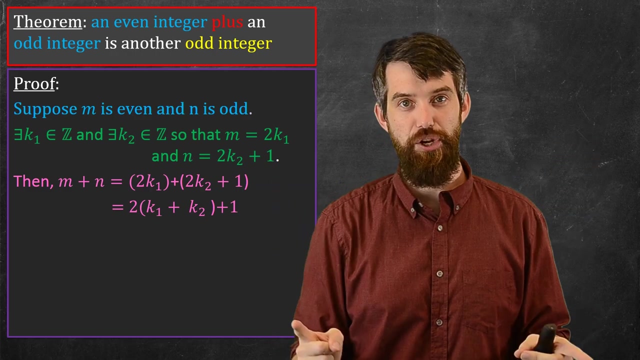 I want the sum of m plus n to be an odd integer. So I want the sum of m plus n to be written as twice an integer plus 1.. Well, it's sort of this. It's written as twice something plus 1.. The something is k1 plus k2.. 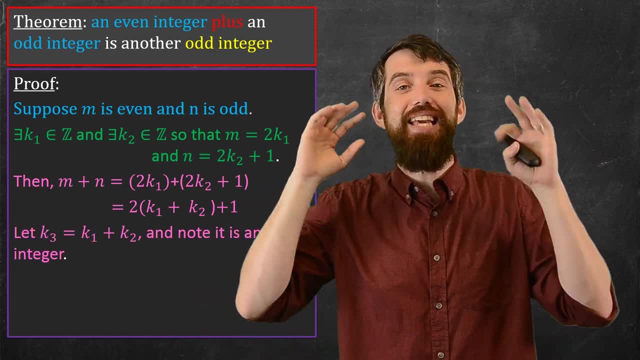 So what I'm gonna do is I'm gonna go and define a third k. I'm gonna define a k3, and the k3 is the sum of the two k's. So I'm gonna go and define a third k. I'm gonna define 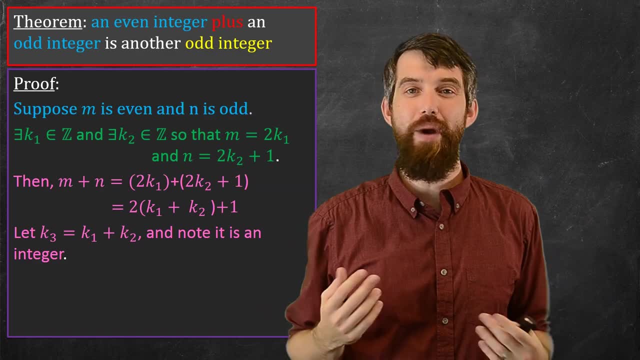 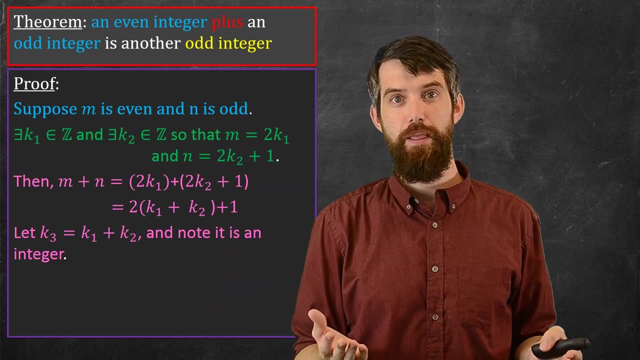 of the k1 and the k2. and, by the way, since k1 was an integer and k2 is an integer and the sum of two integers is an integer, k3 is also an integer. now, why do i like that? well, what have i done here? 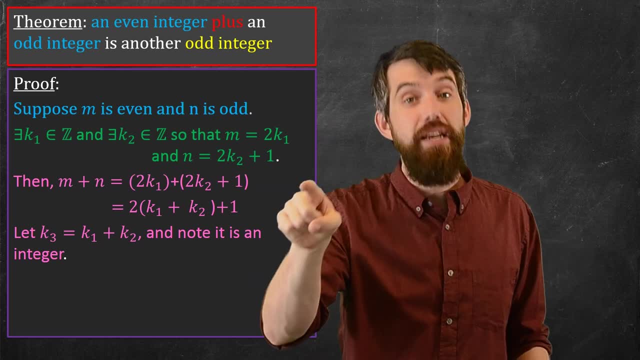 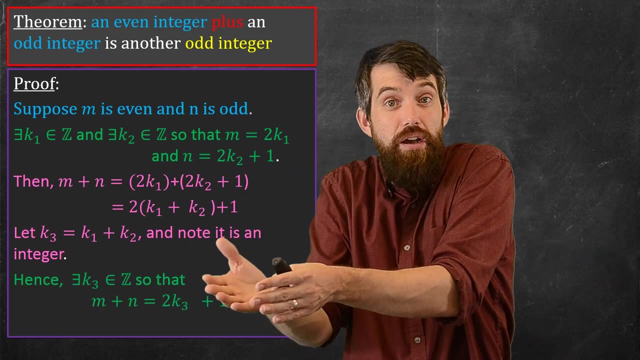 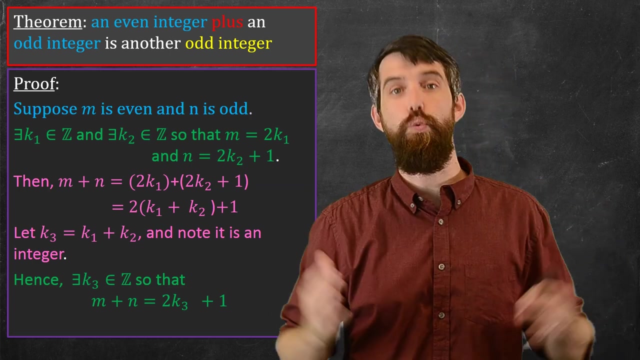 i now i'm in a position to write the definition of the conclusion, that is, i can say that i've got a k3 such that m plus n, the sum of these two things, can be written as twice k3 plus one, and that's just a different way of saying that m plus n is an odd integer. so that's it, that's the. 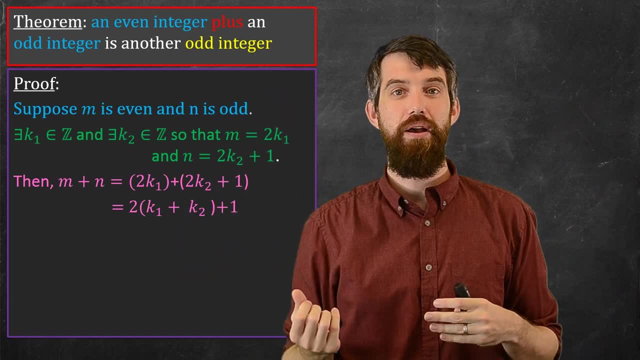 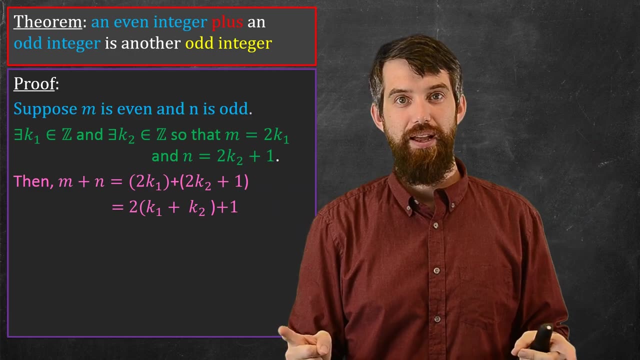 as twice an integer plus 1.. Well, it's sort of this. It's written as twice something plus 1.. The something is k1 plus k2.. So what I'm going to do is I'm going to go and define a third k. I'm going to define: 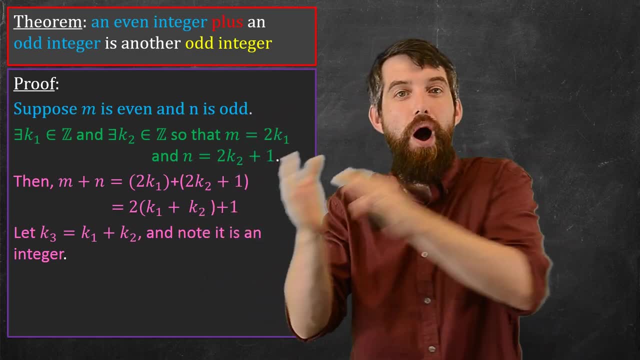 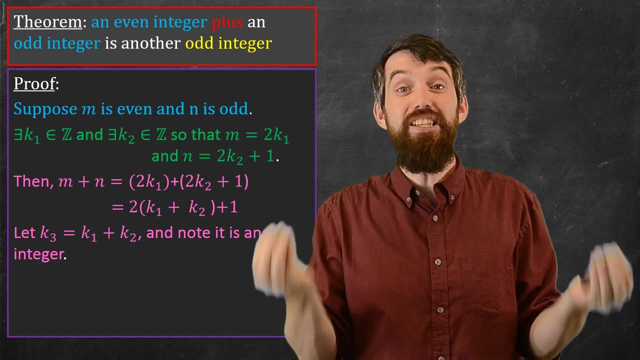 a k3.. k3 is the sum of the k1 and the k2.. And, by the way, since k1 was an integer and k2 is an integer and the sum of two integers is an integer, k3 is also an integer. 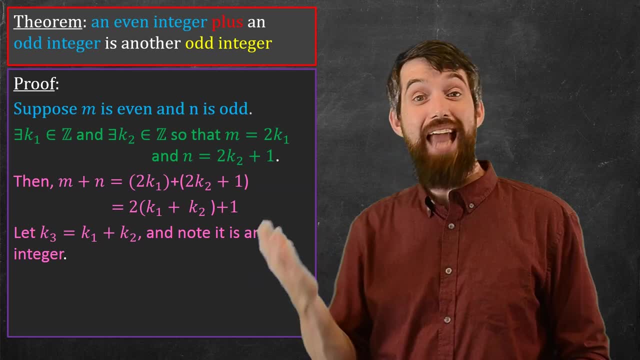 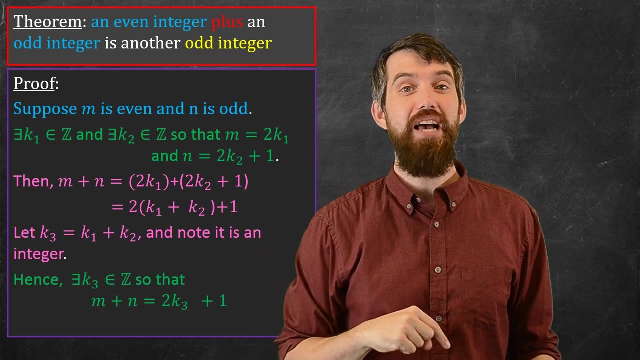 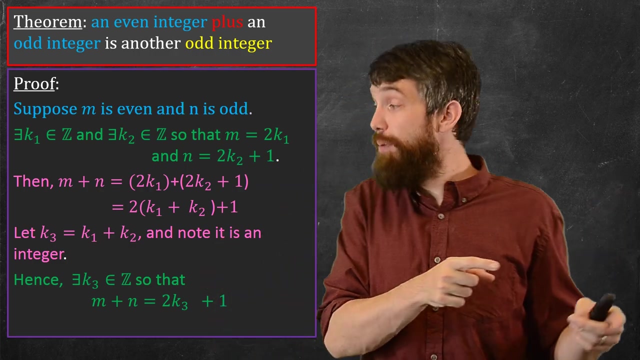 Now, why do I like that? Well, what have I done here? I now am in the position to write the definition of the conclusion, That is, I can say that I've got a k3, such that m plus n, the sum of these two things. 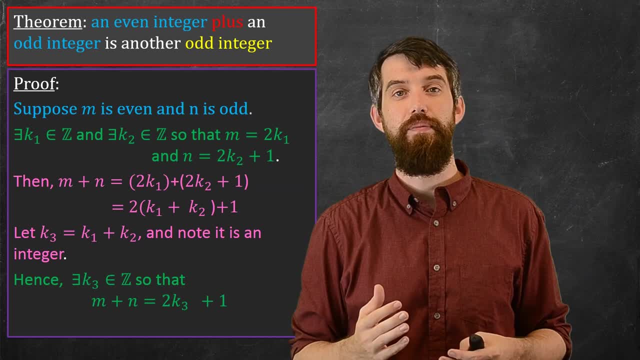 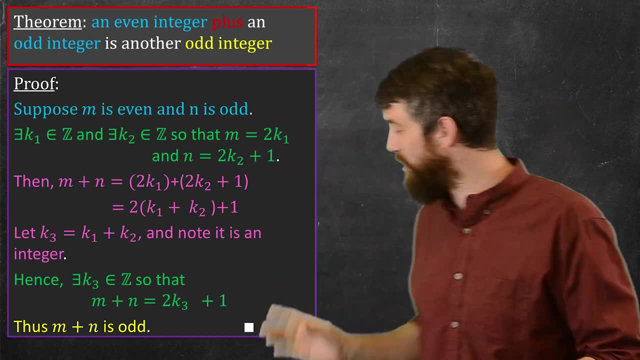 can be written as 2.. twice k3 plus 1.. And that is a different way of saying that m plus n is an odd integer. So that's it. That's the end of my proof, And I can put this little qed box to denote. 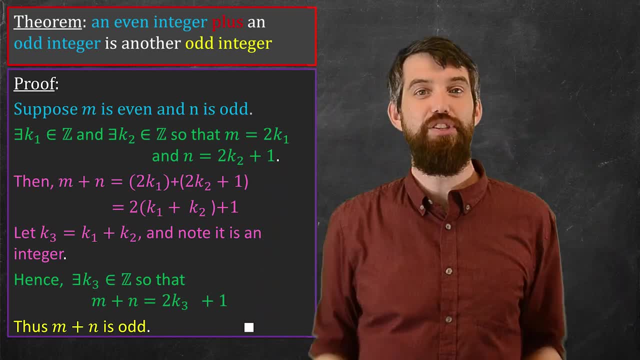 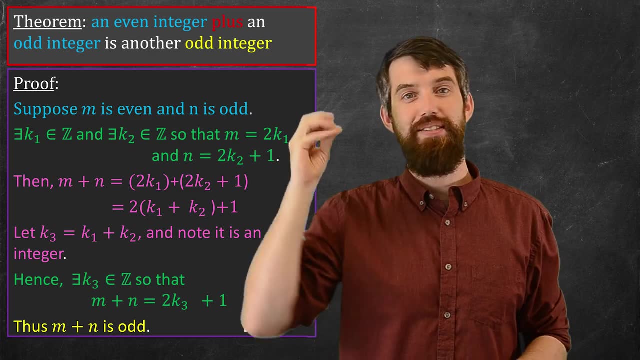 that I'm at the end of my proof. OK, so let's think about the structure of this. Well, we started in the beginning, we've gone to the end. I am now compelled to believe that, indeed, in every scenario, the sum of 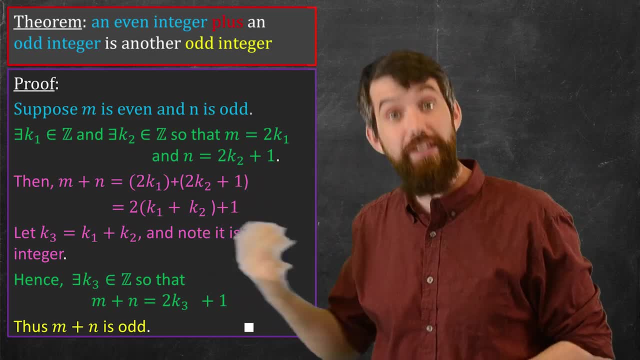 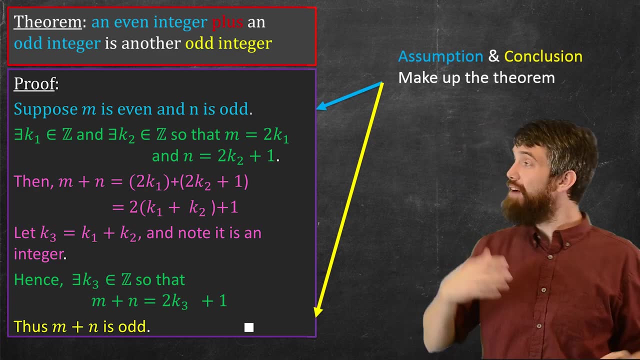 an even and an odd has to be an odd, And this proof is what convinces me of that particular claim. the way it worked was that at the beginning and at the end, what do I have? Well, I have the assumption going down to the conclusion. I began at the beginning, I ended at the end, so that part 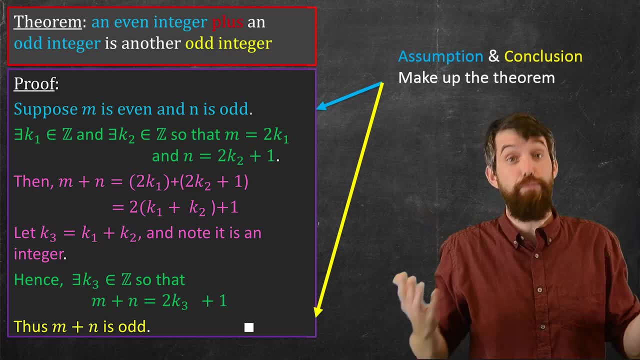 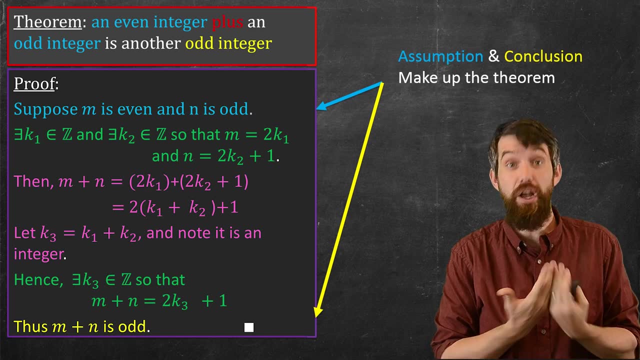 was good, And this should always be the first and last line of any proof that you write. Heck, you can even go and write the end of your proof before you do anything in the middle, if you so choose, because you know where you're trying to go. to is the conclusion: But then I have the green stuff. 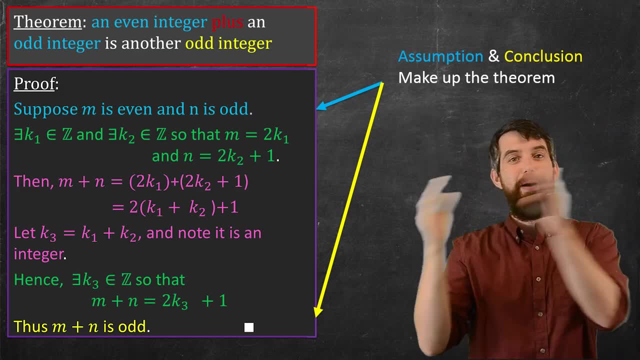 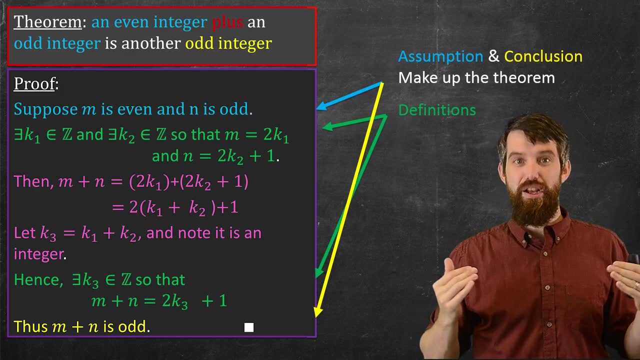 and the green. the first green is the definition of my assumptions and the final one is the definition of my conclusion. So the assumption and the conclusion might be written a little bit vaguely. they might use some math terminology, but when I'm making an actual proof I want to have 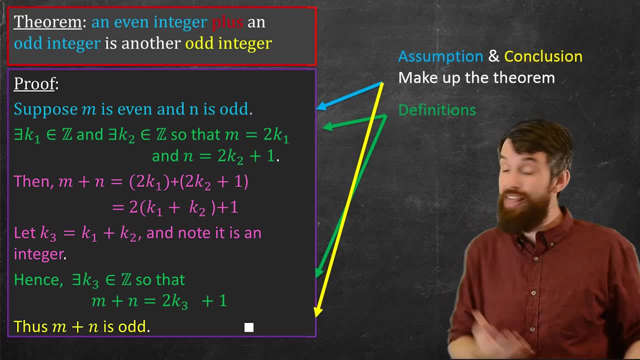 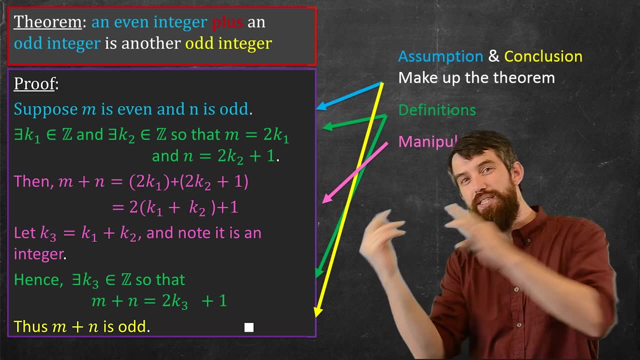 those ideas expressed clearly with formal definitions, and so that's what the green's going to represent. And then the pink stuff in the middle. the pink is my manipulations. In this case, I took a sum, I plugged the definitions in. 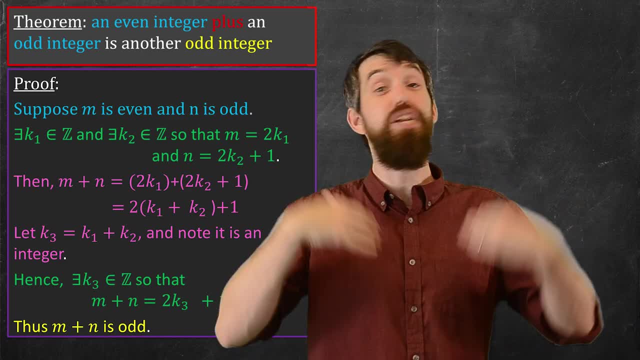 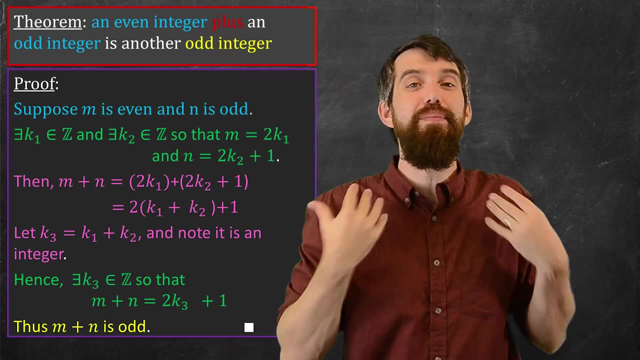 end of my proof, and i can put this little qed box to denote that i'm at the end of my proof. okay, so let's think about the structure of this. well, we've started the beginning, we've gone to the end. i am now compelled to believe that, indeed, in every scenario, the sum of an even 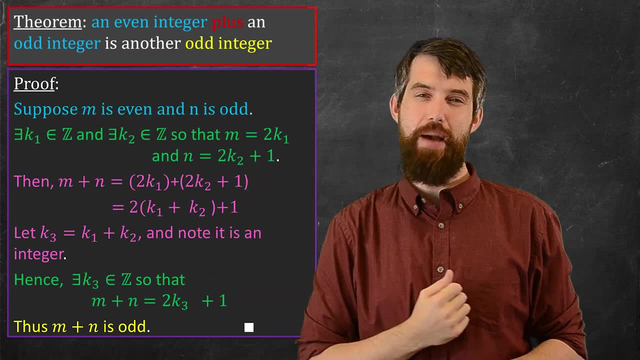 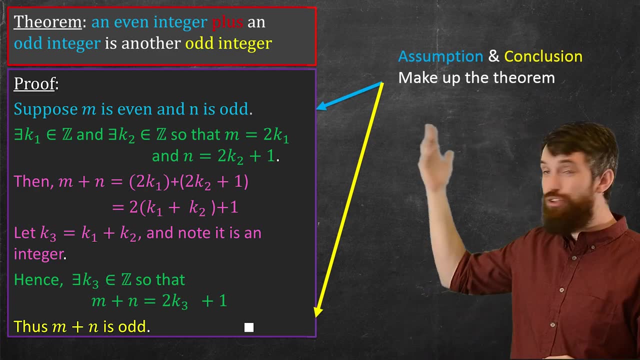 and an odd has to be an odd, and this proof is what convinces me of that particular claim. and the way it worked was that at the beginning and at the end. what do i have? well, i have the assumption going down to the conclusion. i began at the beginning, i ended at the end, so that part. 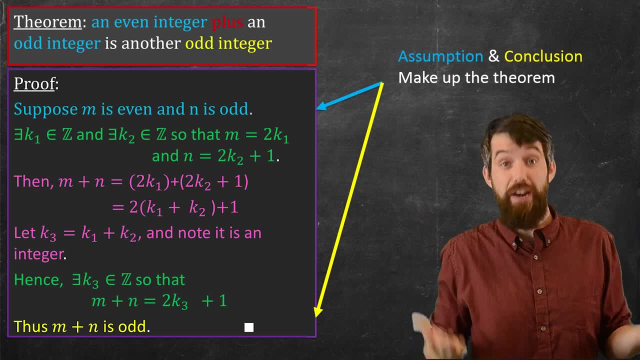 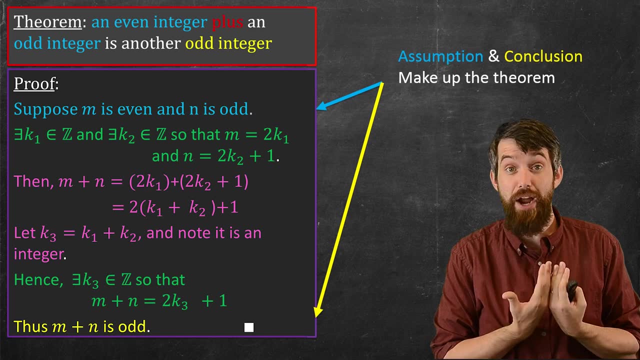 was good, and this should always be the first and last line of any proof that you write. heck, you can even go and write the end of your proof before you do anything in the middle, if you so choose, because you know where you're trying to go. to is the conclusion. but then i have the green stuff. 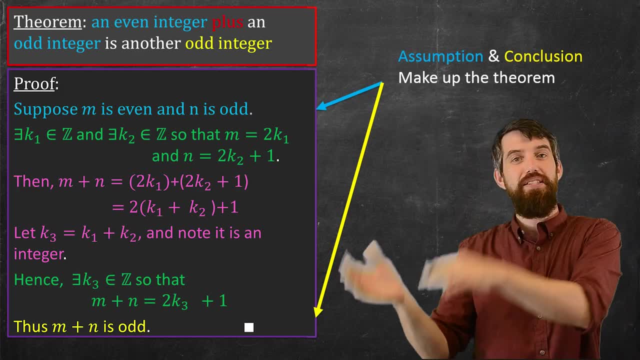 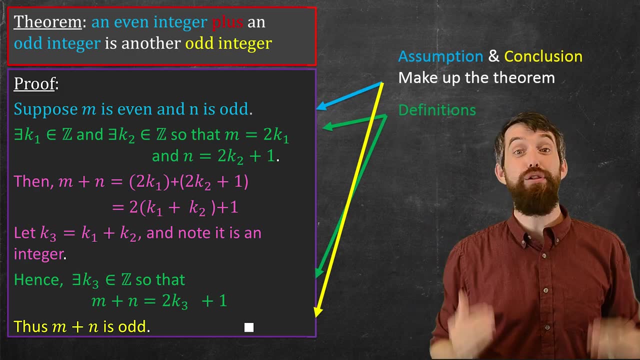 and the green. the first green is the definition of my assumptions and the final one is the definition of my conclusion. so the the assumption and the conclusion might be writing a little bit vaguely. they might use some math terminology, but when i'm making an actual proof i want to. 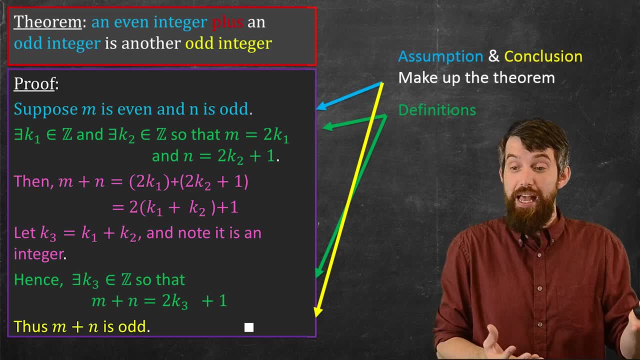 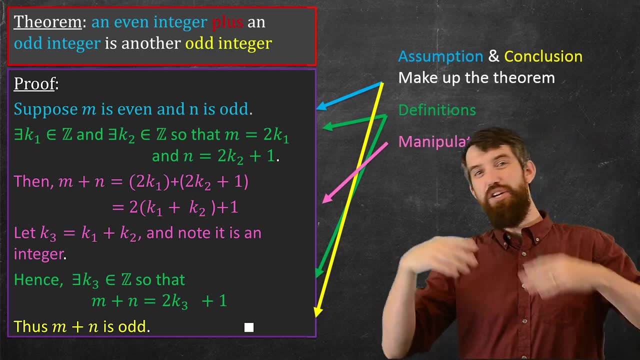 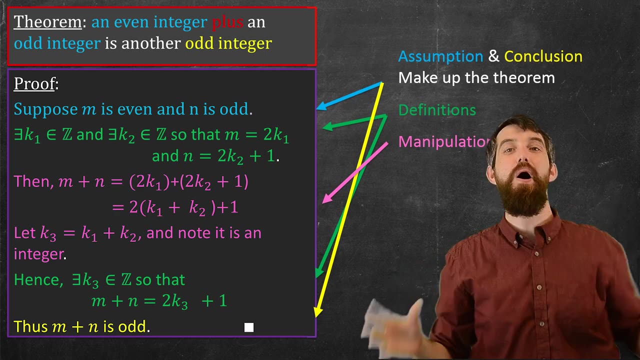 have those ideas expressed clearly with formal definitions, and so that's what the greens can represent. and then the pink stuff in the middle. the pink is my manipulations. in this case i took a sum, i plugged the definitions in, i factored out the two, i defined this k3. that's sort of the body of the proof. so this basic structure that i have here, 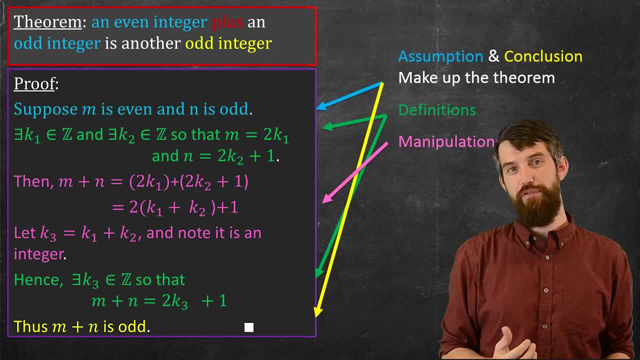 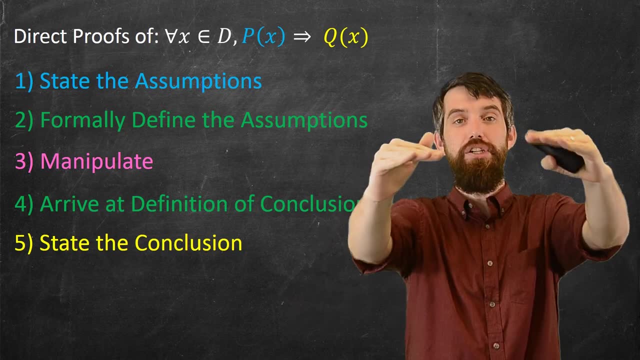 it repeats itself in proof after proof after proof, that you're going to have this five step process, in fact, where you state the assumption, you state the definition of the assumption, you do a bunch of manipulations, you get to the definition of the conclusion and finally you state: 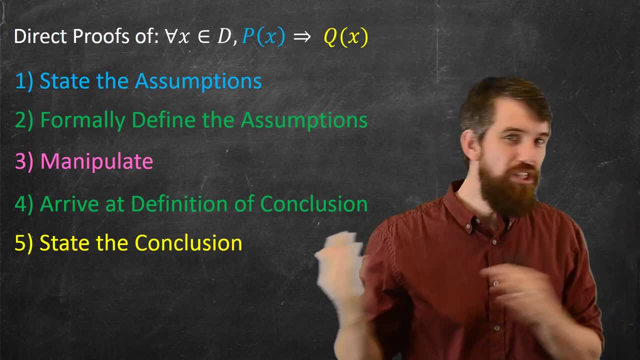 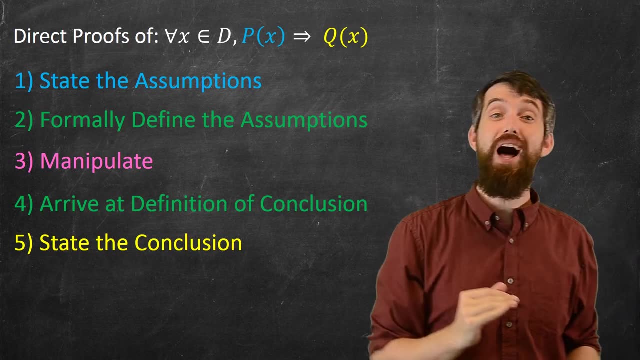 the conclusion. now the actual definitions change to proof to proof and the actual assumptions and conclusions change proof to proof. but steps one, two, four and five are all kind of a bit for free. you can sort of write them down and if you know what your definitions are, you you can get most of 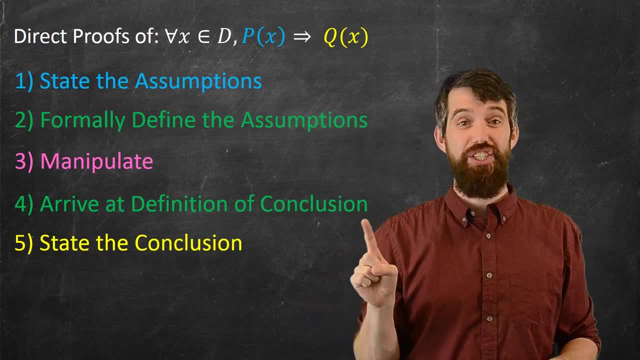 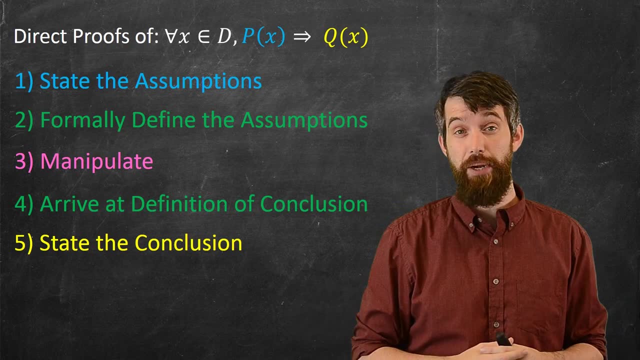 the structure of the proof. what's the hard part is the manipulations, and that changes is different for every single proof. in this case, we had a relatively simple manipulation, but in some proofs it can be very challenging. final point about this, in terms of the structure of the proof: 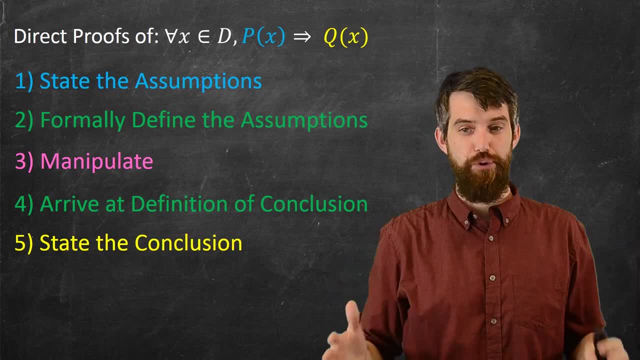 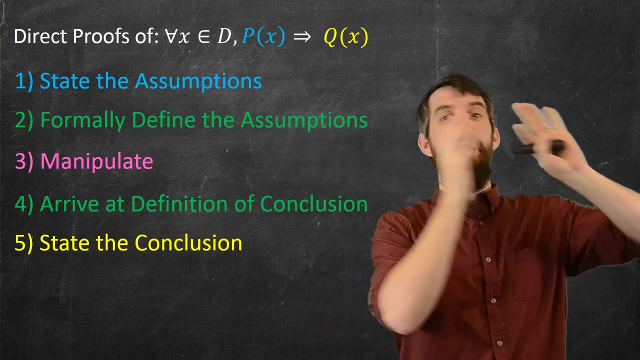 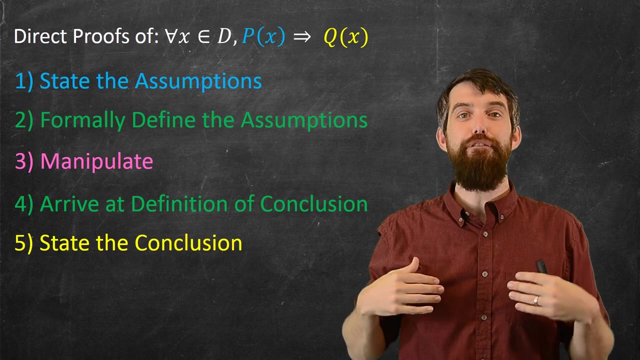 so let's talk about proofs first of all. proofs are proofs of the claim where you're saying for every value in some domain, you're saying the p of x's imply the q of x's and you're starting with your assumption p and you're going towards your conclusion q. this is a for all style statement. 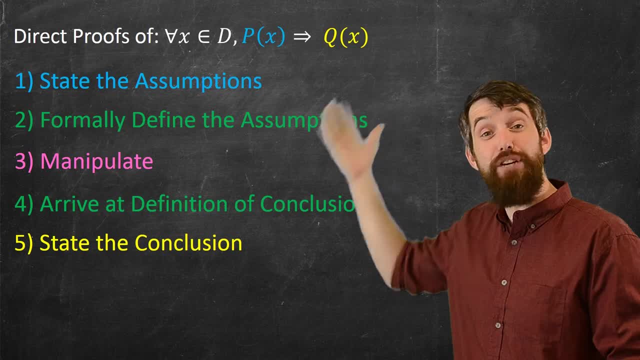 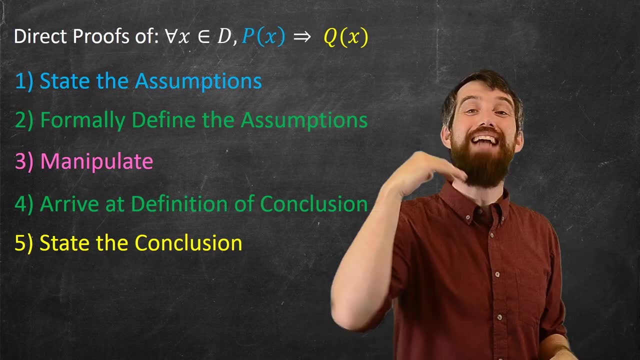 and there's other types of proofs out there. first of all, you might have a different order to how you prove things. for example, you could prove things by contrapositive or contradiction. we're going to learn them later. you can have existent or non-existent proofs. you can prove things by 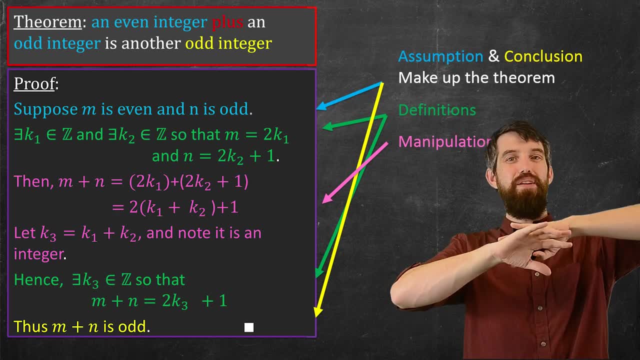 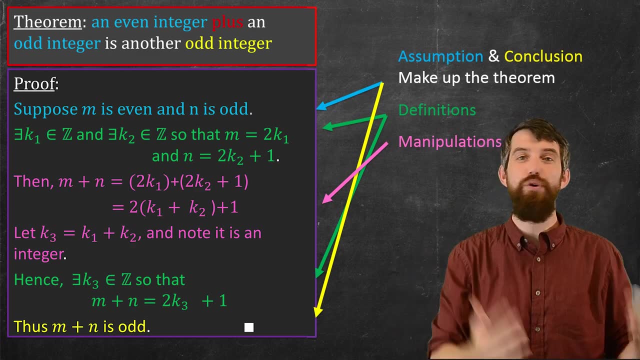 I figured out what the green was and I figured out what the green was. Factored out the two, I defined the k3, that's sort of the body of the proof. So this basic structure that I have here, it repeats itself in proof after proof, after proof that you're going. 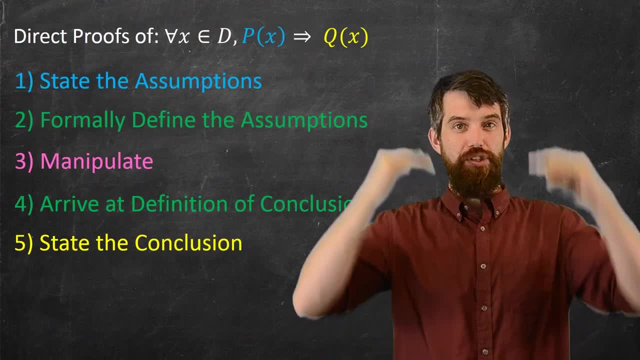 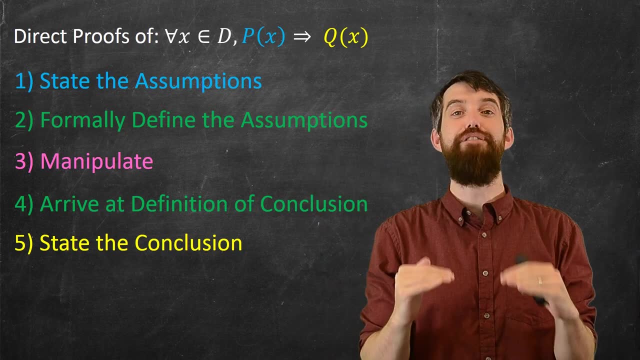 to have this five-step process, in fact, where you state the assumption, you state the definition of the assumption, you do a bunch of manipulations, you get to the definition of the conclusion and finally you state the conclusion. Now the actual definitions change to proof, to proof. 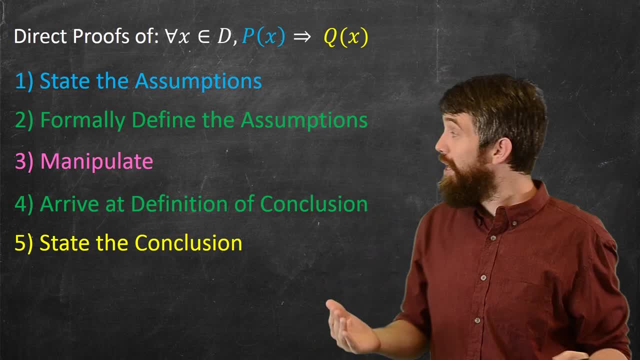 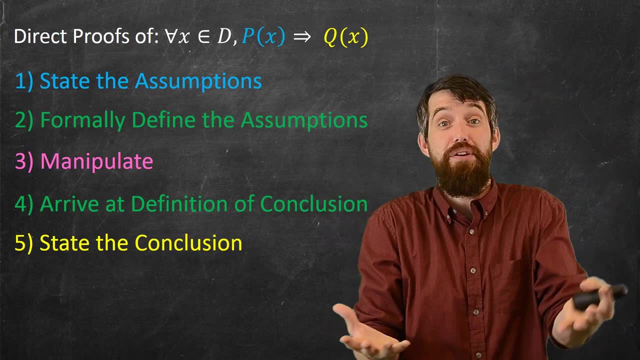 and the actual assumptions change to proof to proof and the actual assumptions change to proof to proof. But steps one, two, four and five are all kind of a bit for free. You can sort of write them down and if you know what your definitions are, you can get most of the structure of 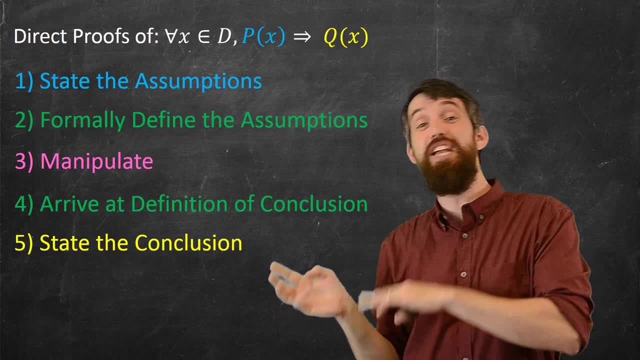 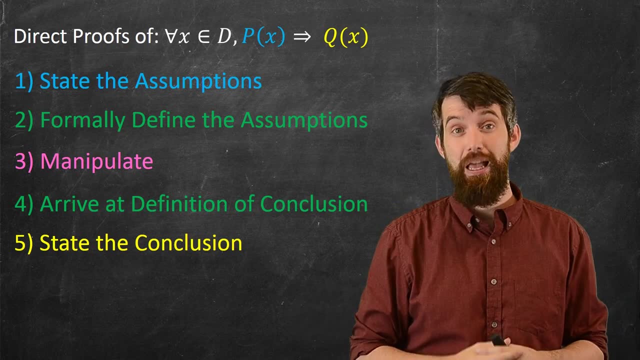 the proof. What's the hard part is the manipulations, and that change is different for every single proof. In this case we had a relatively simple manipulation, but in some proofs it can be very challenging. Final point about this: introduction to proofs. This is for so-called direct proofs, Proofs. 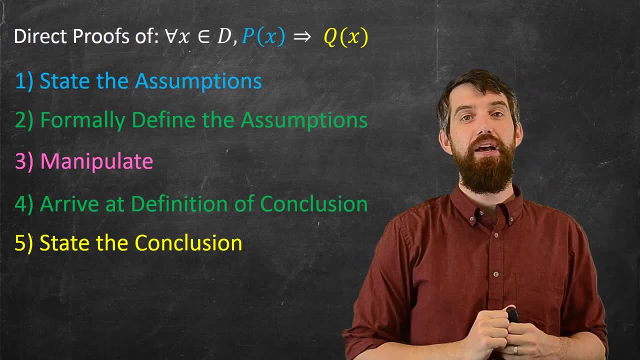 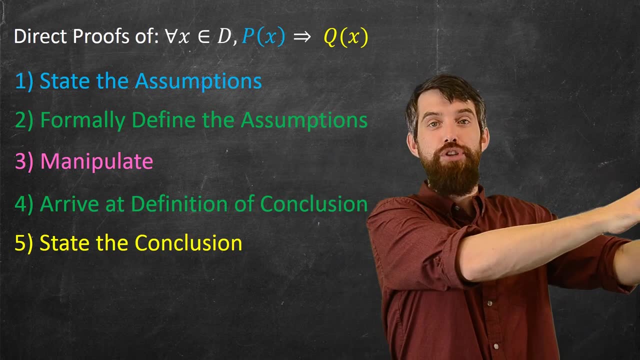 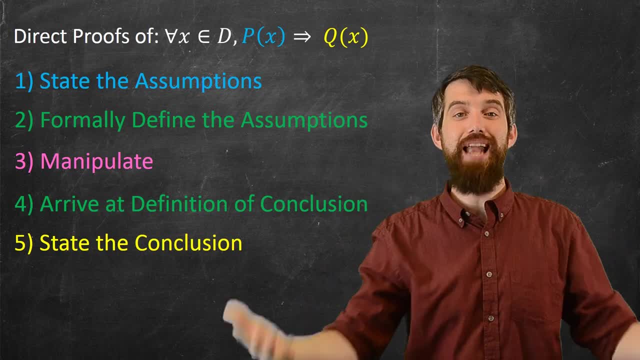 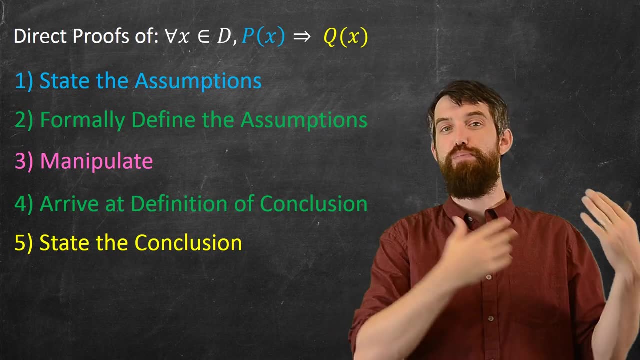 q. This is a for-all style statement And there's other types of proofs out there. First of all, you might have a different order to how you prove things. For example, you could prove things by contrapositive or contradiction. We're going to learn them later. You can have 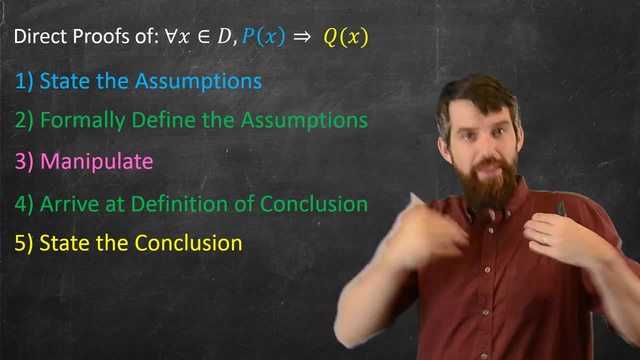 existential proofs, opposed to these sort of for-all proofs. But in this case it's a for-all proof because we're saying: for every value in some domain, you're saying the p of x's, imply the q of x's, And you're starting with your assumption p and you're going towards. 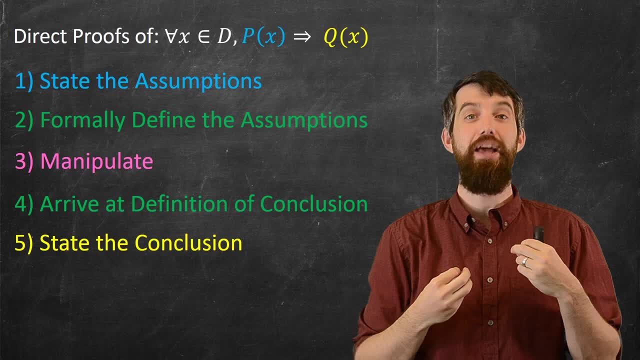 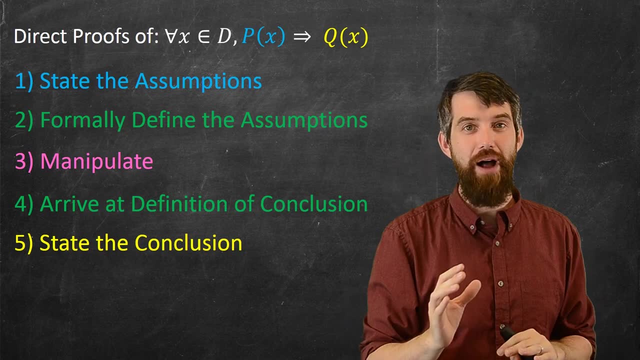 every possible m that's even, and every possible n that's odd. Then your sum is going to be odd as well. So this five-step method for direct proofs, I hope, will serve you very well, And you're going to have a whole bunch of different types of proofs that are using this basic structure.